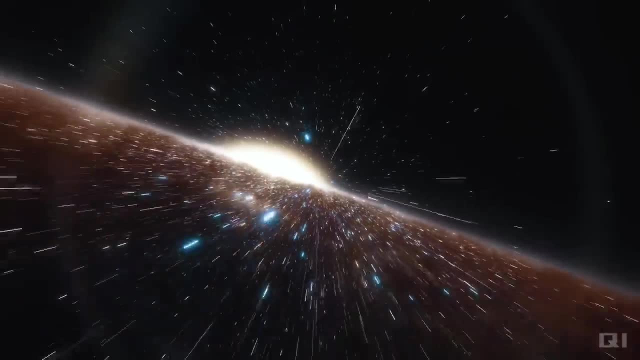 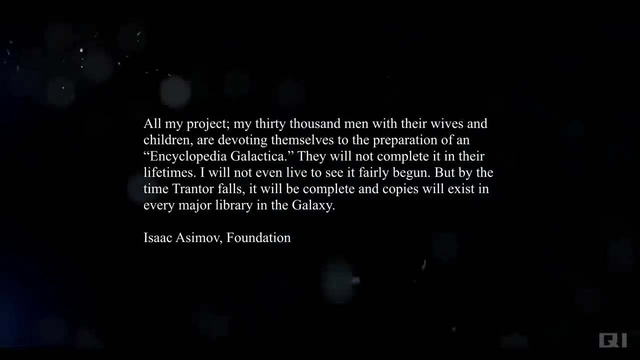 knowledge of all mankind, in the hope that doing so could shorten the interregnum which would follow the collapse of the empire. All my project, my 30,000 men with their wives and children are devoting themselves to the preparation of the entire empire. 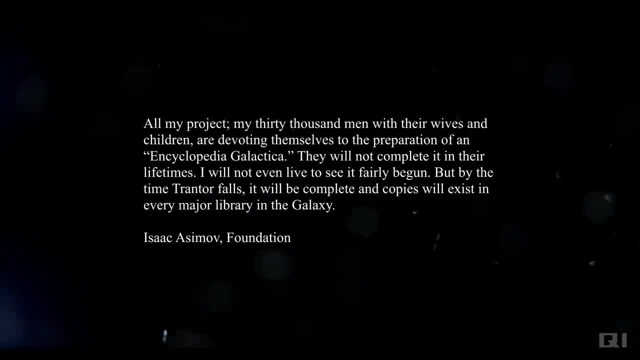 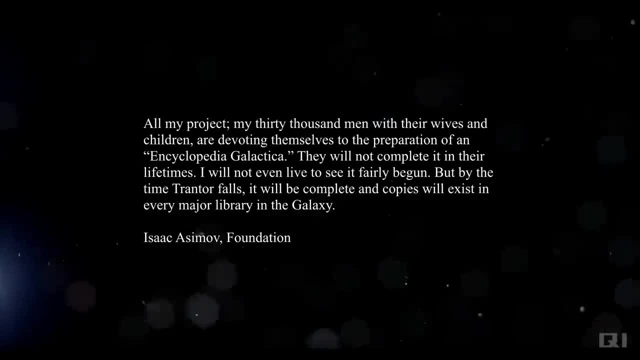 The foundation would be based on the foundation of an Encyclopedia Galactica. They will not complete it in their lifetimes. I will not even live to see it thoroughly begun. but by the time Trantor falls it will be complete and copies will exist in every major library. 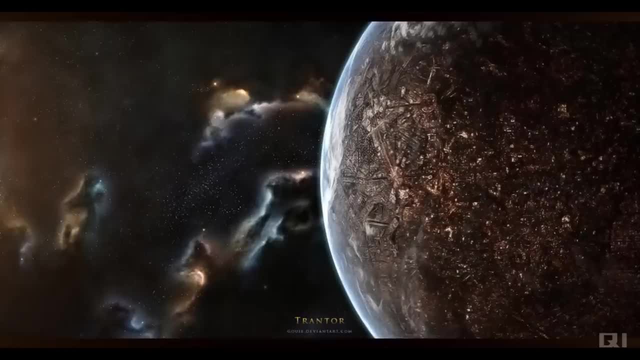 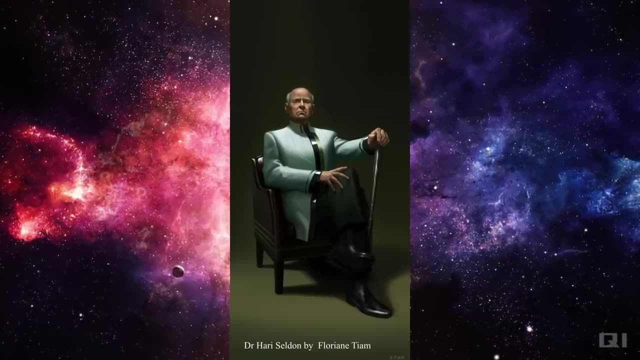 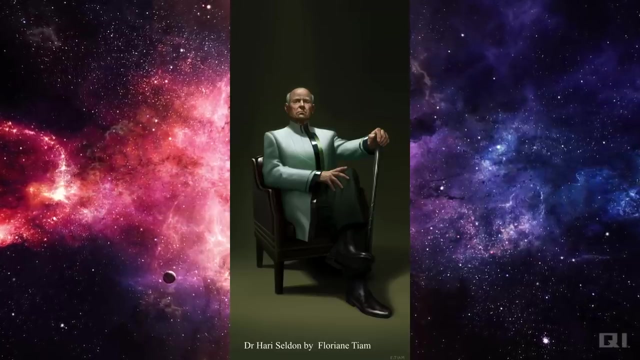 in the galaxy. Though it had been initially stated that the foundation existed solely to create the Encyclopedia Galactica, it is revealed a third of the way through the first book, 50 years after its initial creation, that the Encyclopedia was. encyclopedia is not the true purpose of the Foundation at all. Harry Seldon had left a 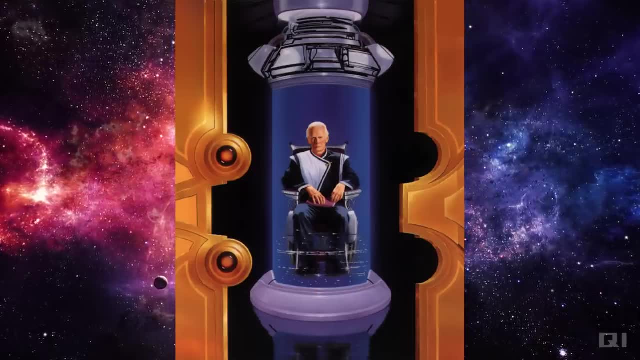 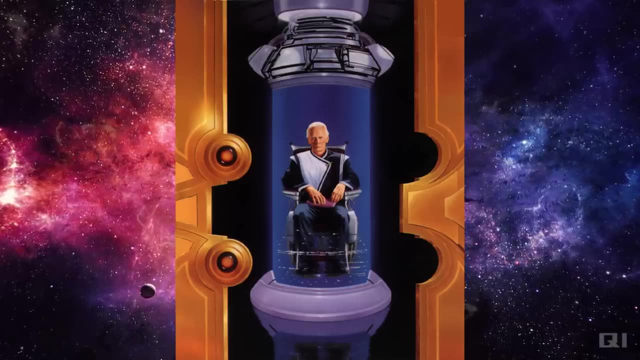 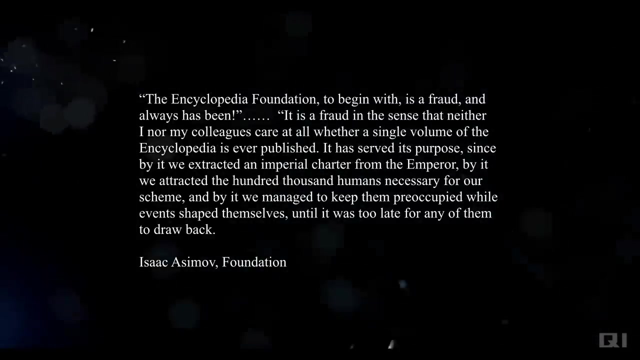 vault on Terminus. It was set to open on a specific date in which the pre-recorded holograms of Seldon would appear to address the Foundation. The vault opens and a hologram of him reveals the truth: The Encyclopedia Foundation, to begin with. 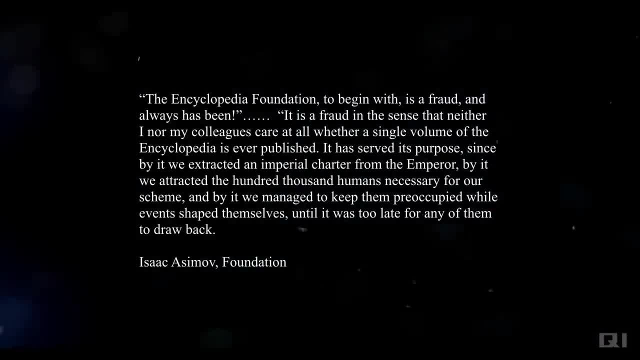 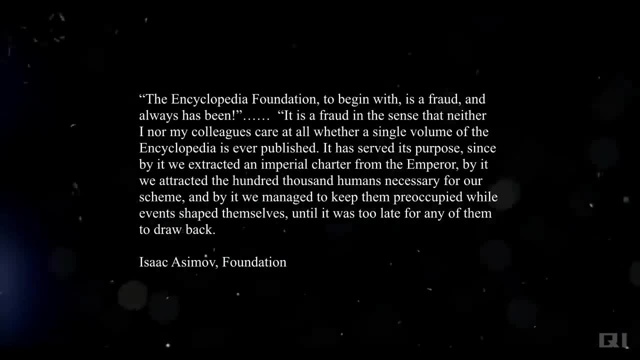 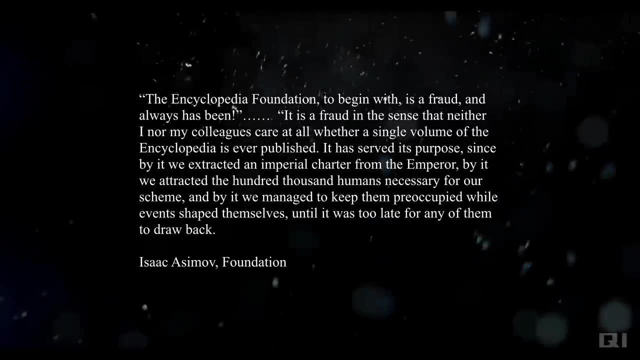 is a fraud and always has been. It is a fraud in the sense that neither I nor my colleagues care at all whether a single volume of the Encyclopedia is ever published. It has served its purpose since by it we extracted an Imperial Charter from the Emperor. by it we attracted 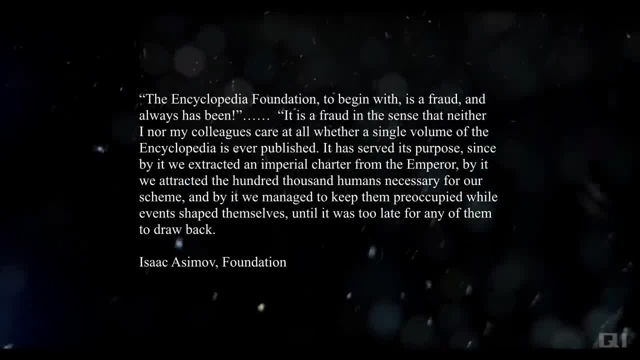 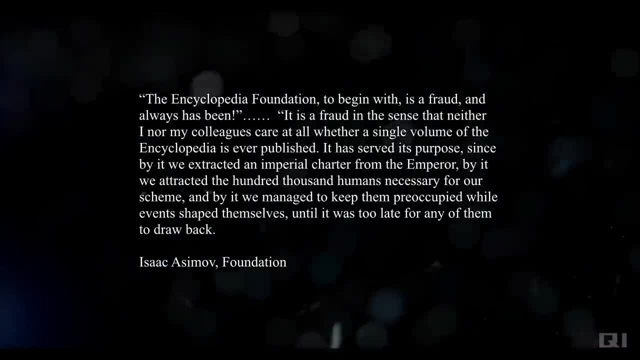 the 100,000 humans necessary for our scheme, and by it we managed to keep them preoccupied while events shaped themselves, until it was too late for any of them to draw back. Harry Seldon tells them that the path for the Foundation is inevitable. They will be faced with a series 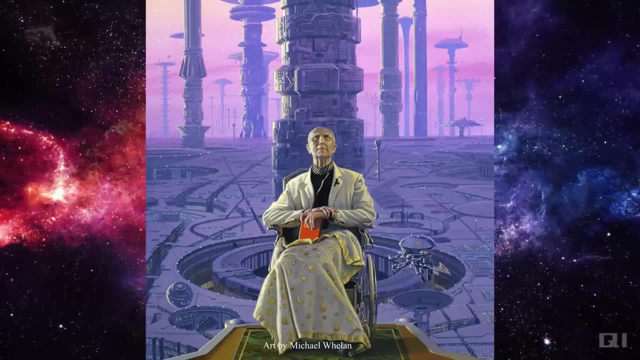 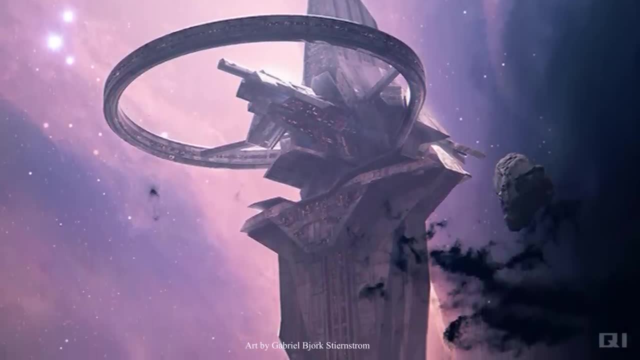 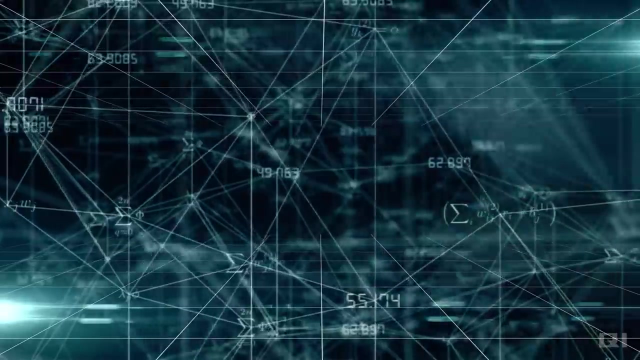 of crises That he himself had predicted through psychohistory. He tells them that in each crisis they will be forced along a singular path due to the circumstances set in place. The path they will take will be past, laid out in Harry Seldon's psychohistory calculations. As I said, psychohistory- 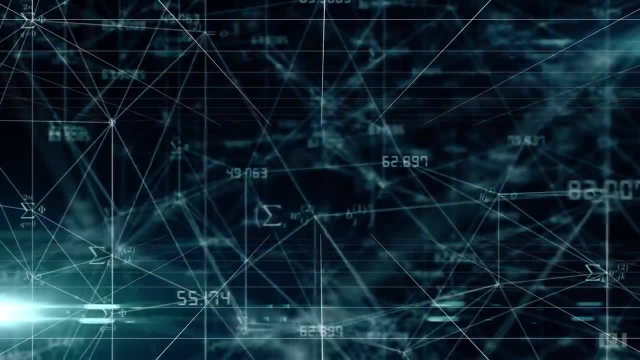 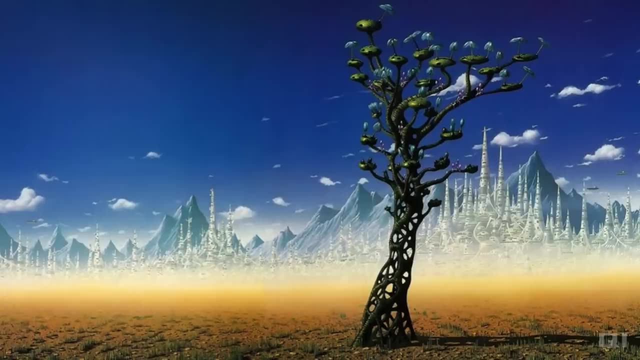 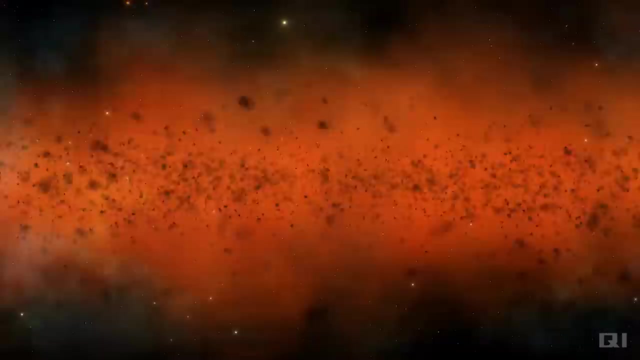 could predict human psychology at mass over long distances of time, As it develops over the centuries. the Foundation is met with crisis after crisis, just as Seldon had predicted. Each time, his pre-recorded hologram appears to advise them. Later in the series, however, Seldon's plan is shaken with the arrival of the Mule, The